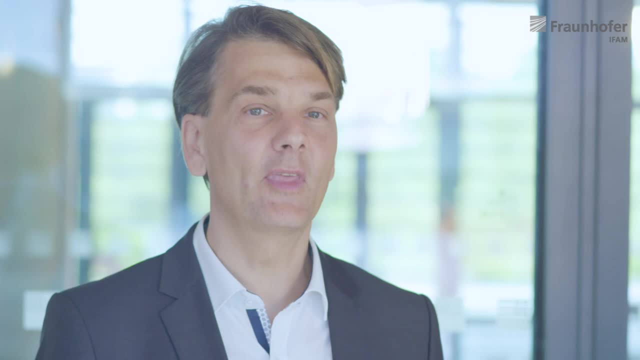 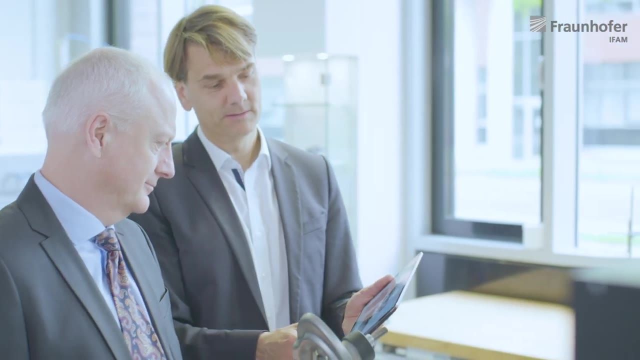 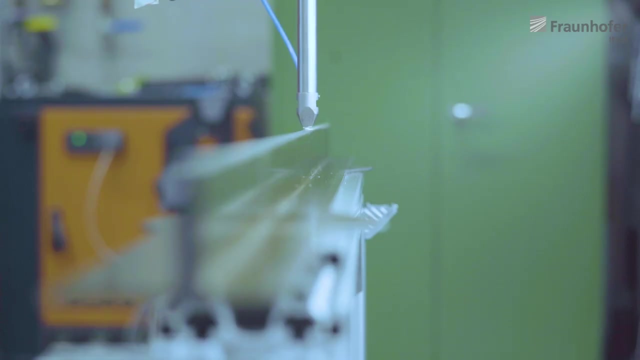 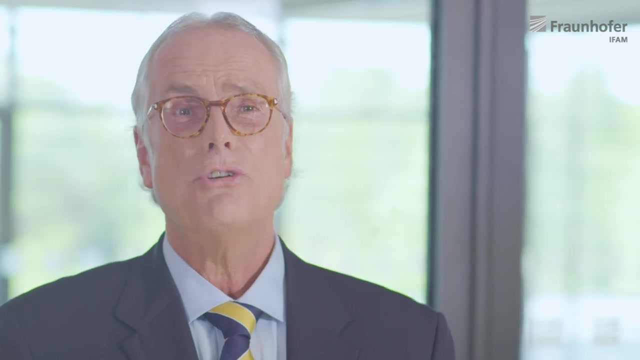 compliant, reproducible and economic bonding. That is a challenge we face. Our customers range from craftsman's businesses to large international corporations. Our customers benefit from our innovative strengths: speed and experience. Safety is an essential precondition to achieve confidence in a technology. 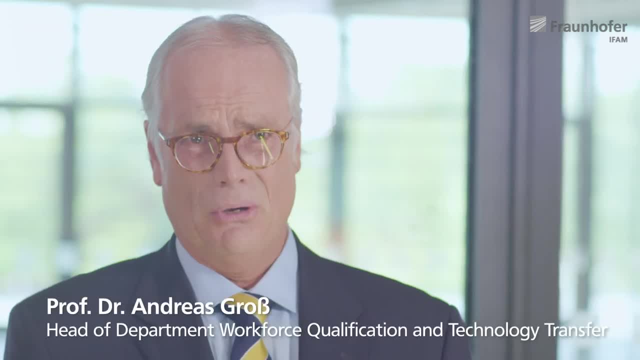 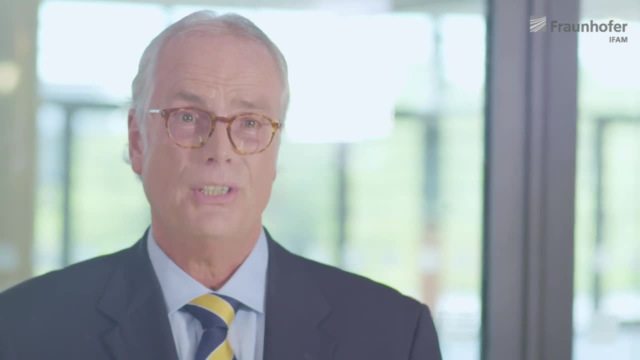 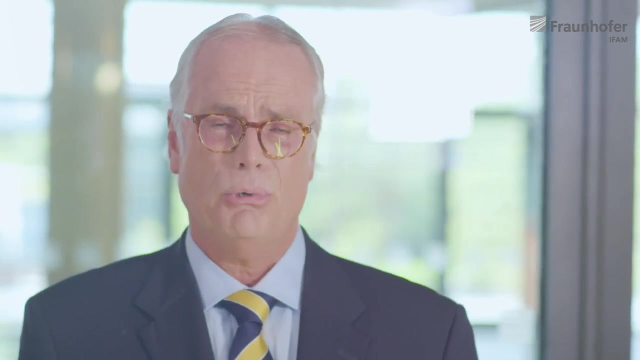 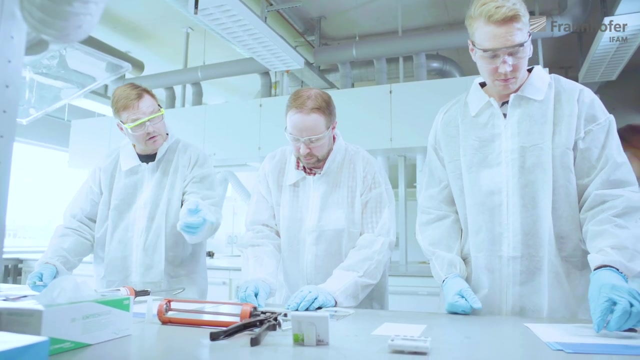 Adhesive bonding is a very complex process. There are a lot of quality influencing factors which have to be considered And therefore it is necessary that the people who use adhesives and who are using adhesive bonding technology are. competent will mean qualified on each topic which has to be regarded. That will mean we need a 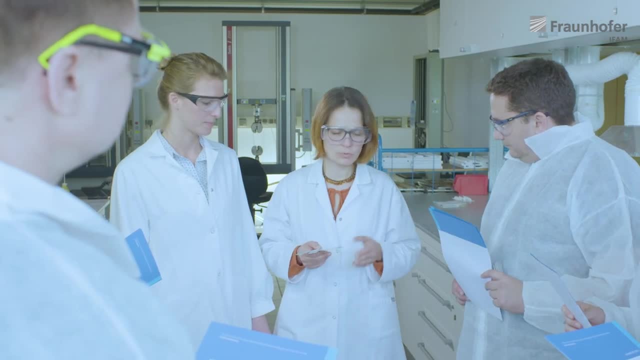 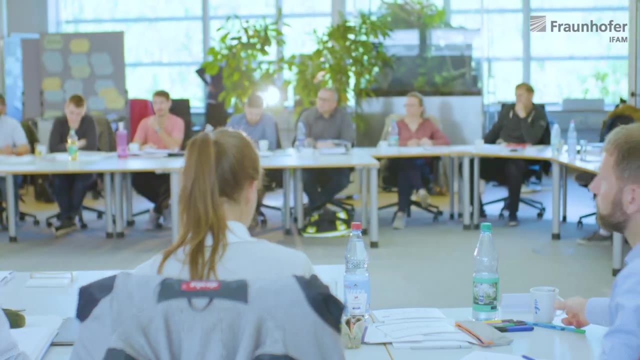 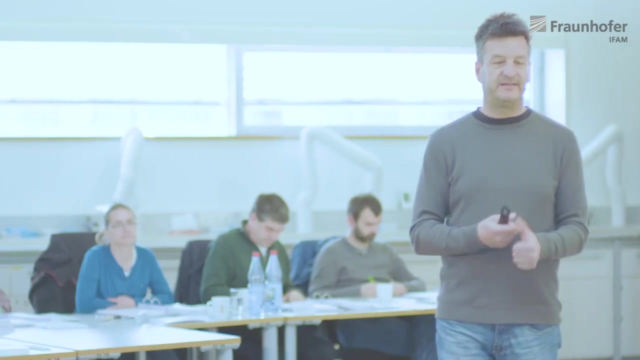 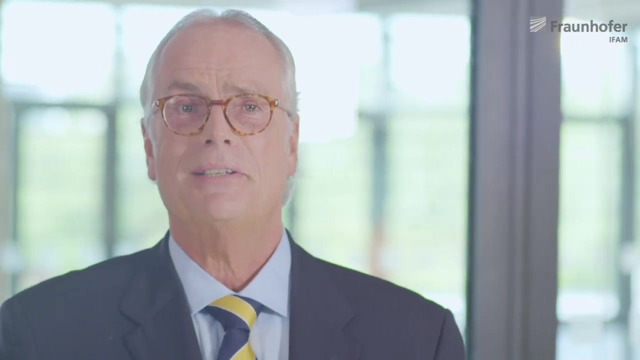 tactical view on adhesive bonding technology and on each adhesive bonding process. step A: personnel-certified workforce qualification makes your competence comparable world wide. That the workforce qualification is implemented and carried out world wide- yes, this makes us a little bit proud. The implementation of quality standards relation to professional and instructional education, sih, which includes the artificialkkea technology, can be useful to the beginner standardised workforce. Thank you very much. 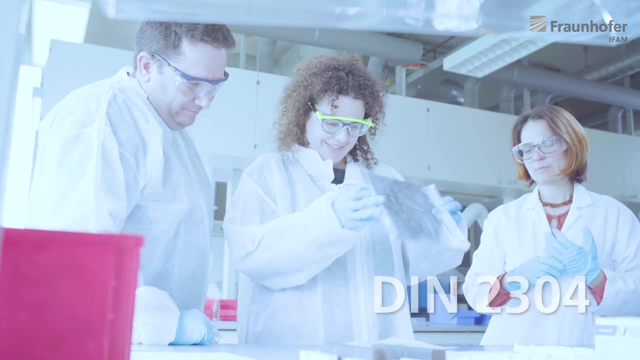 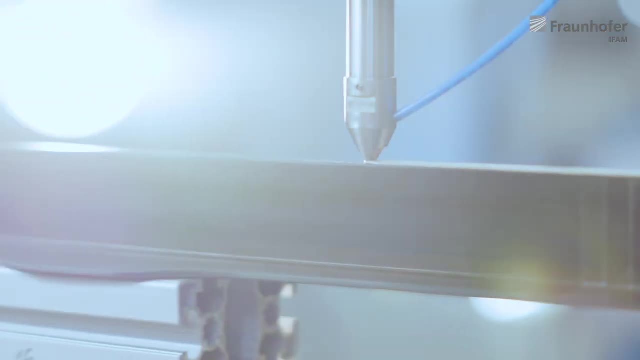 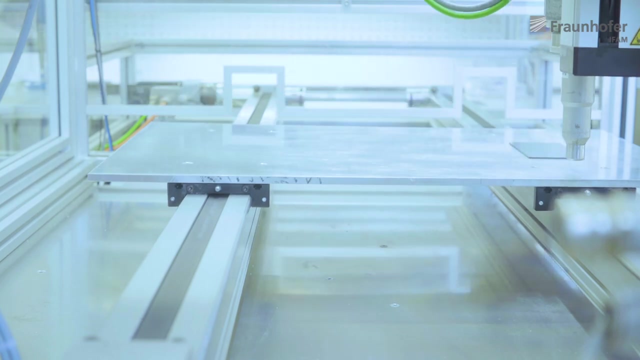 Adhesive bonding processes according to DIN 2304 and DIN 6701, are key steps. In close cooperation with industrial partners. we are heavily involved in writing international standards. We work industry-oriented and result-oriented. We are independent problem solvers. 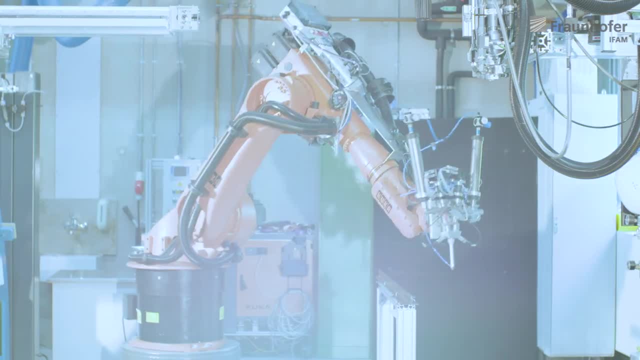 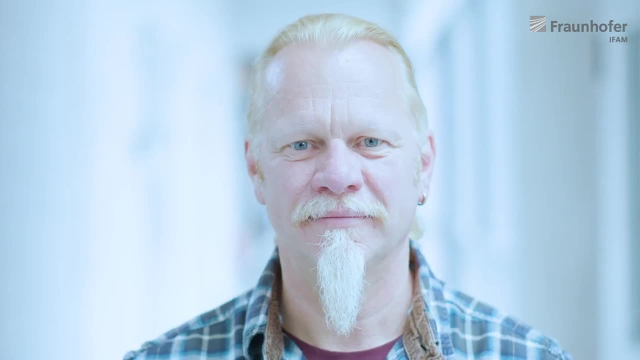 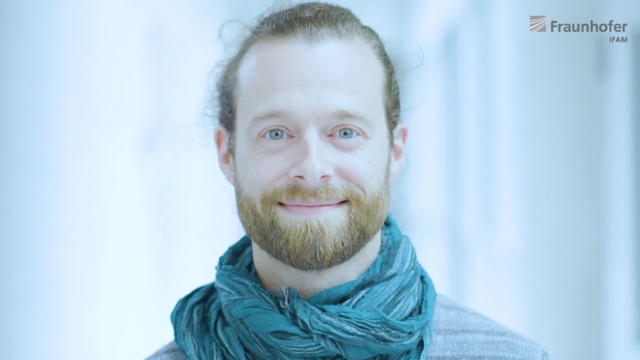 Adhesive bonding will be the leading joining technology of the 21st century. Together we already achieved a lot and want to continue to convince with our innovative concepts. We believe in social responsibility to make the technology accessible for all markets, applications and industries. We are fully committed to take up this challenge.